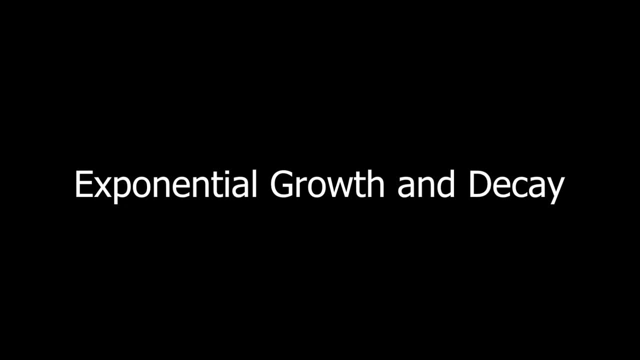 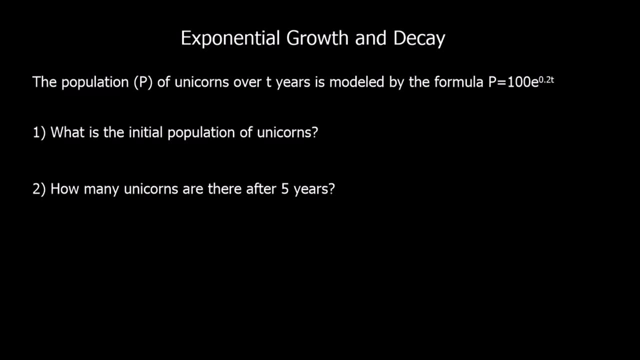 This video is about exponential growth and decay. Here we've got a question. The population of unicorns over t years is modelled by the formula given. What is the initial population of unicorns? So the initial population is going to be where t equals zero. So we're 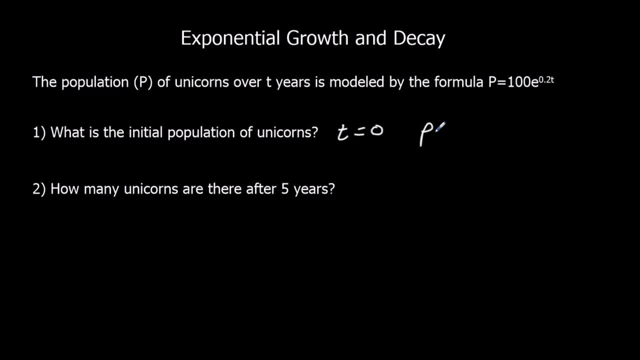 just going to substitute t equals zero in here, So that will give us p equals 100e to the power of zero, point two zeros, And well, anything to the power of zero is going to be one. so that's just going to leave us with 100.. So the initial population is 100. 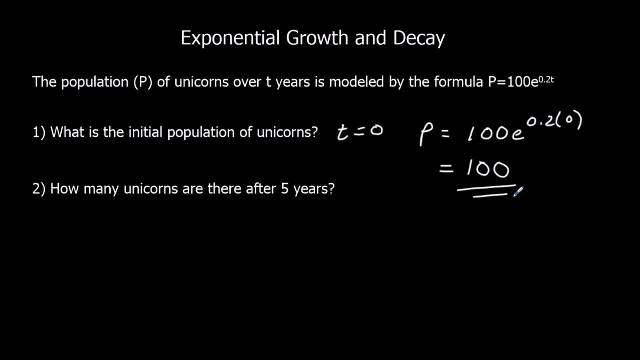 unicorns. How many unicorns are there after five years? So when t equals five years, t equals five. So again we're just going to substitute in: t equals five, So p equals 100e to the power of zero point two times five. So we can just type that into the calculator. 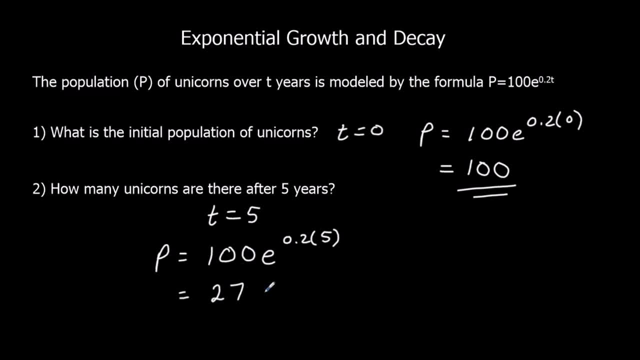 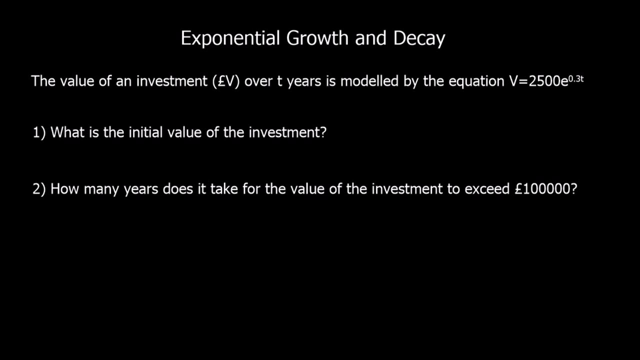 and we get out an answer of two hundred and seventy one point eight, But to the nearest whole unicorn, two hundred and seventy two unicorns. The value of an investment over t years is modelled by the equation given: What is the initial value of the investment? So again, initial value, that's when t equals zero. 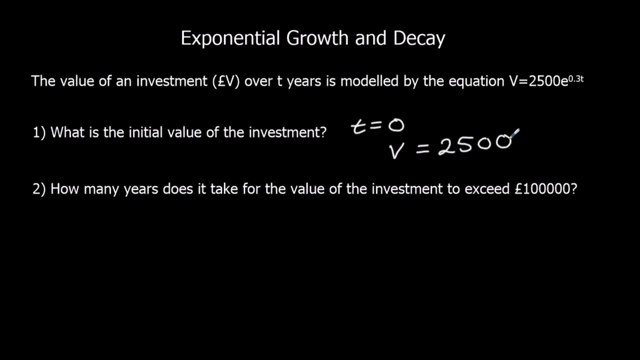 So we substitute in: t equals zero. Anything to the power of zero is going to be one. So we're left with two thousand five hundred pounds. How many years does it take for the value of the investment to exceed one hundred thousand? So we've got, if we work out where the investment is equal to one hundred thousand, and we'll 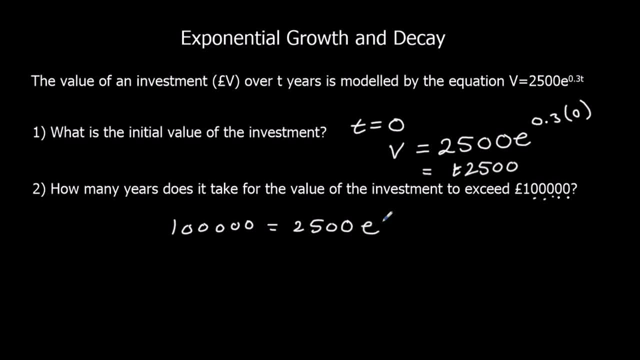 be able to see how many years it takes to exceed it. So we're going to solve an equation using e. So the first step: we're going to divide one hundred thousand by two thousand five hundred, which is 40. So 40 equals e to the power of zero point three t. Now to 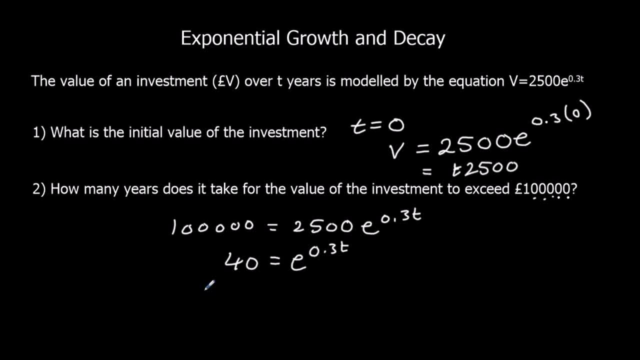 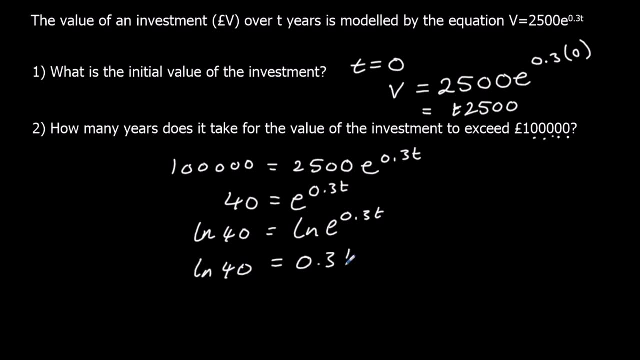 get rid of e, we're going to apply ln to both sides. So ln 40 equals ln e to the power of zero, point three. t ln e is going to cancel, So ln 40 equals 0.3 t. So t if we divide both sides by 0.3, t is ln 40 divided by 0.3.. 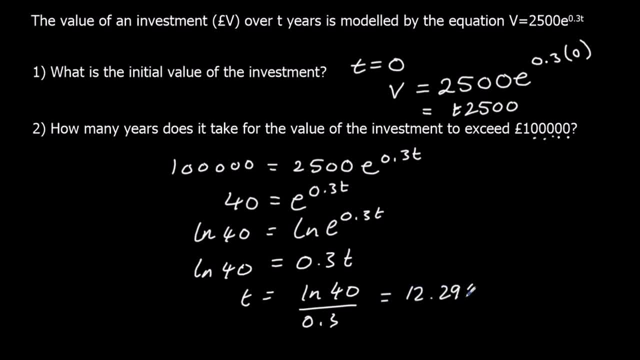 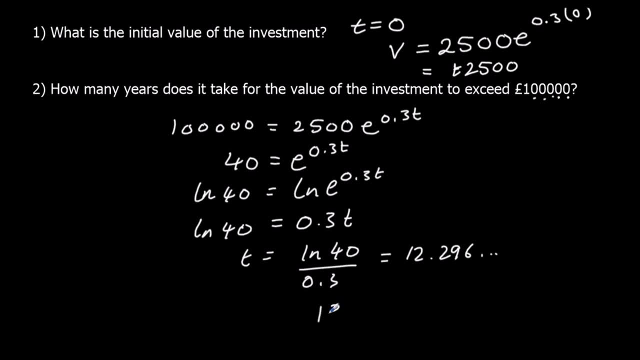 And so that gives us an answer of twelve point two, nine six. So how many years to exceed a hundred thousand? It's going to take thirteen years, Because it's equal to a hundred thousand after twelve point something years. So thirteen years to exceed a hundred thousand. 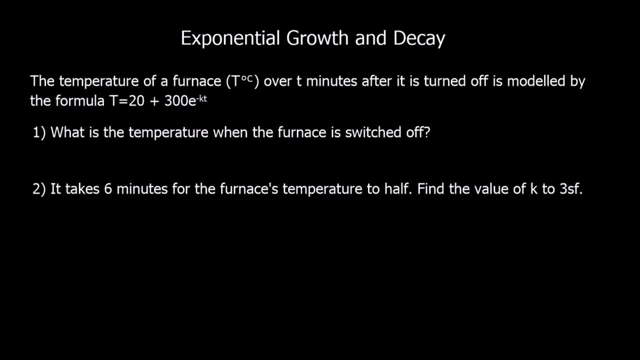 The temperature of a furnace over t minutes is modelled by the formula given. What is the temperature when the furnace is switched off? So the initial temperature. so where t equals zero, We've got little. t equals zero. There's a big T as well in this question. 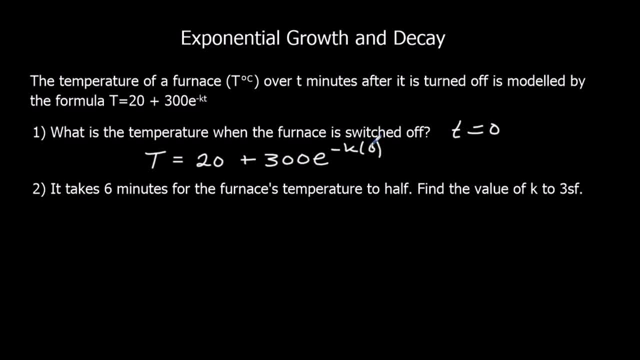 E minus k times zero. So again, n to the power of zero is going to be one. So we're left with twenty plus three hundred, So three hundred and twenty degrees Celsius. It takes six minutes- so t equals six- for the furnace's temperature to happen. It takes six minutes for the furnace's 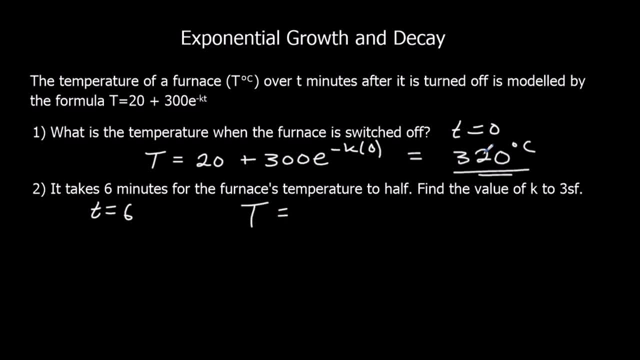 temperature to half. So the temperature big T is half of the original temperature. so a hundred and sixty Find the value of k. So we're going to substitute these in. So one sixty equals twenty plus three hundred e to the power of minus k times six. So let's take twenty off both sides. 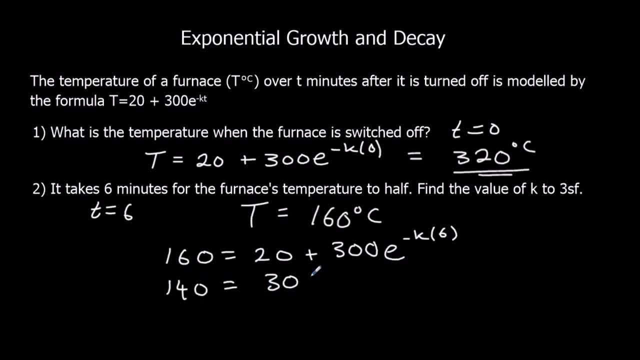 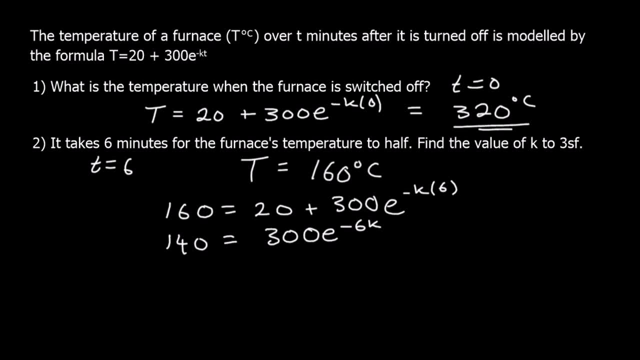 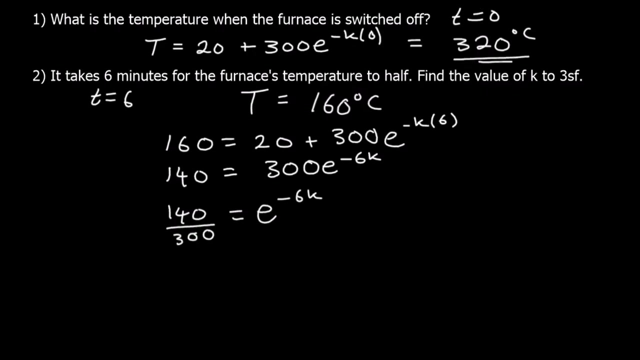 So a hundred and forty equals three hundred, equals three hundred. e to the power of minus six k. Divide both sides by three hundred, So we're left with one forty over three hundred equals e to the power of minus six k. To get rid of e, we're going to apply ln to both sides. So ln one hundred and forty over three. 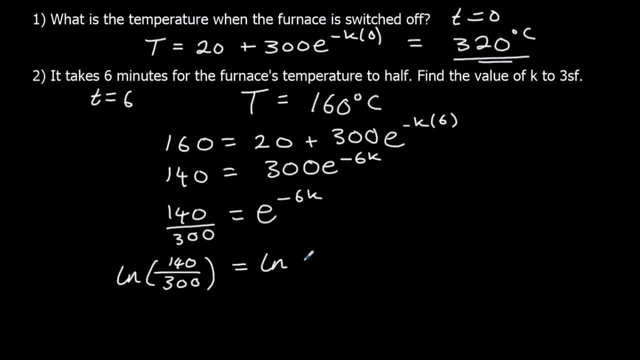 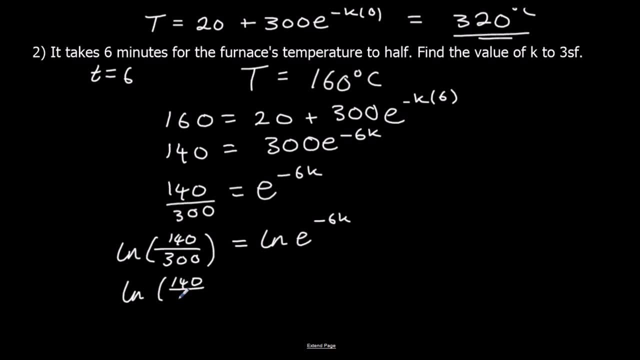 hundred equals ln e minus six k ln e is going to cancel, So that's just minus six k left And we're going to divide by minus six, So that'll give us k equals ln one forty over three hundred. Of course that would cancel, but we can just. 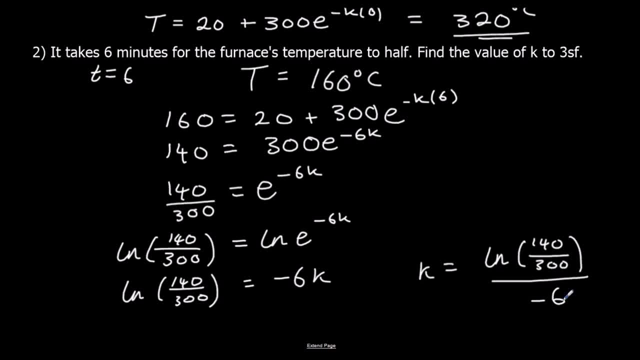 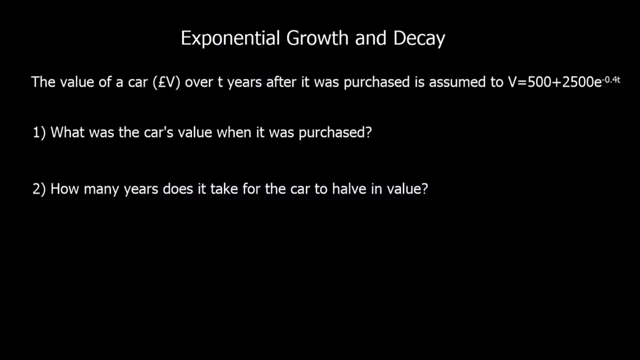 type it into the calculator. Divide by minus six And we get to three significant figures: Zero point one, two, seven And finally, if you want to pause the video, give it a go and then I'll go through the answer after. 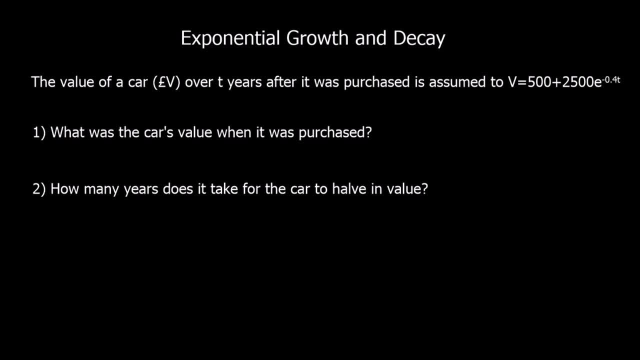 So we've got the value of a car over t years After it was purchased. is the formula given? So what was the car's value when it was purchased? So that's when t equals zero. So that'll be. v equals five hundred plus two thousand five hundred e to the power of minus. 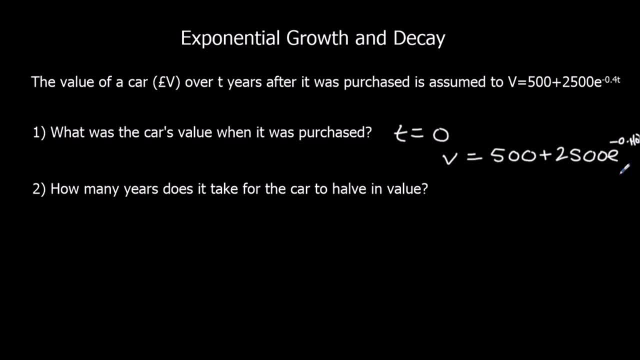 zero point four times zero. Anything to the power of zero is going to be one. So five hundred plus two thousand five hundred three thousand pounds, How long does it take? How many years does it take, for the car to half in value? 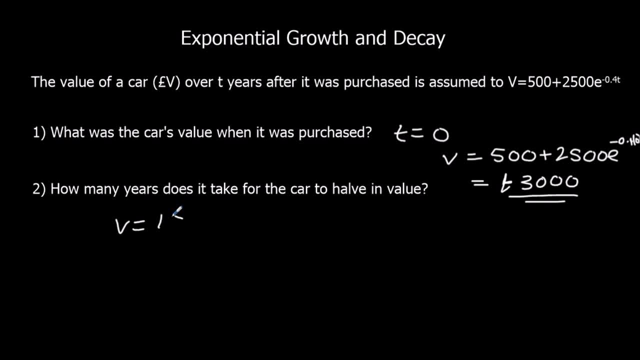 So if it was half the value v would be one thousand five hundred. So one thousand five hundred equals five hundred plus two thousand five hundred e minus zero point four t. So if we take five hundred off both sides, So one thousand equals two thousand five hundred e to the power of minus zero point four t.